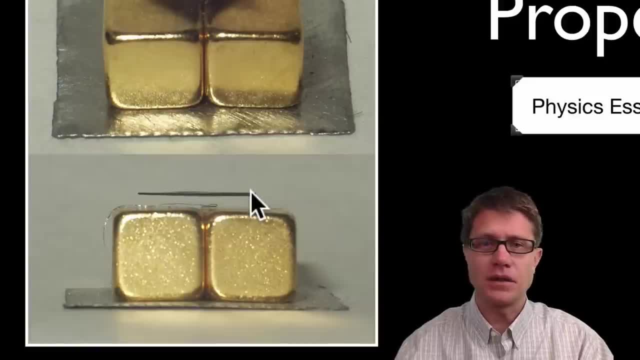 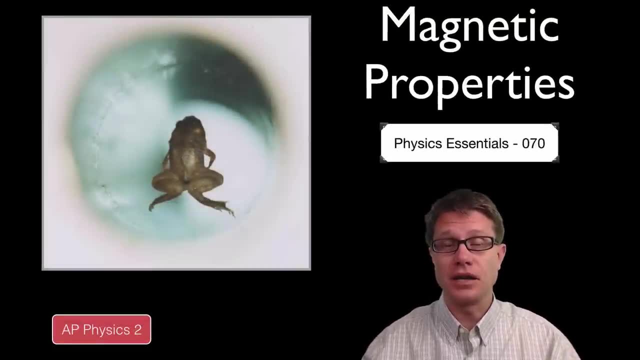 of these magnets. Now you are diamagnetic as well, And that means that if we were to put you in a magnetic field, like they did with these frogs, you will actually be pushed away by the magnetic field lines And you will actually levitate there. Now they have. 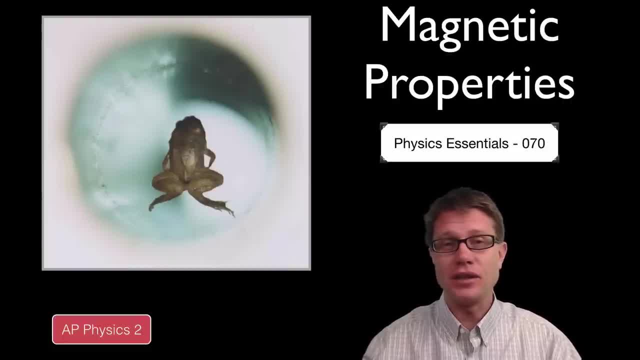 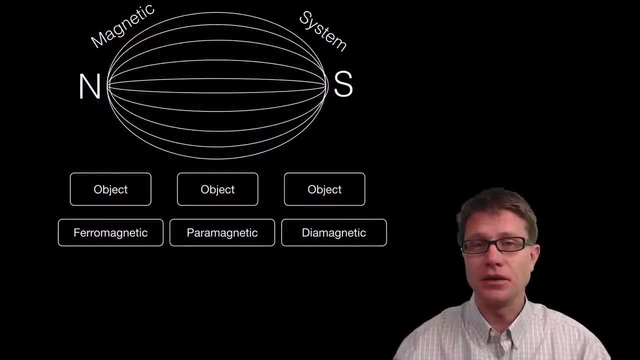 not done humans yet, but they have done frogs and they have done mice, And it is a way that we could kind of study how we respond to weightlessness. And so if you take objects and place them inside a magnetic field, they are going to respond in one of three ways, And they are 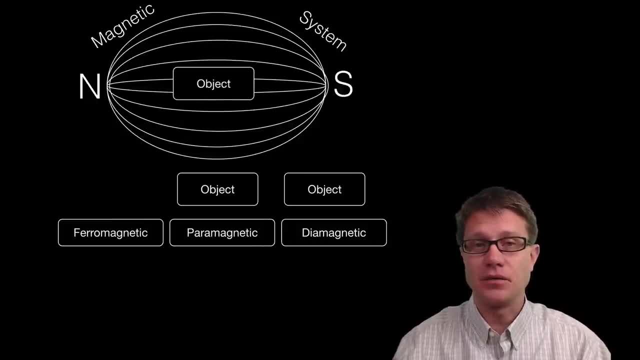 if you are ferromagnetic material and we put you inside a magnetic field, the little electrons and the atoms and the domains will start to align to the electromagnetic fields and it will make a magnet of its own with a north and a south pole And it will make 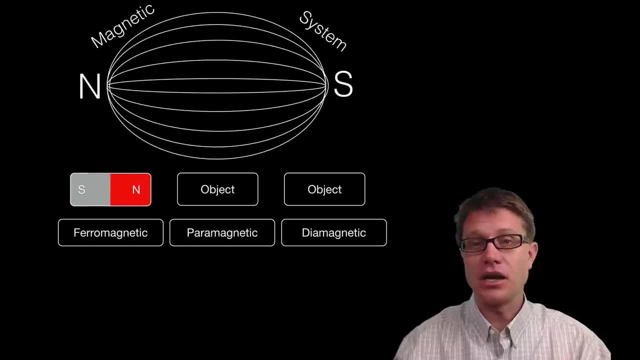 a permanent magnet. That means if we pull it out it is going to stay magnetized And that is because we have aligned these domains inside the object itself. Now, if you take material that is paramagnetic and we put it inside a magnetic field with really strong 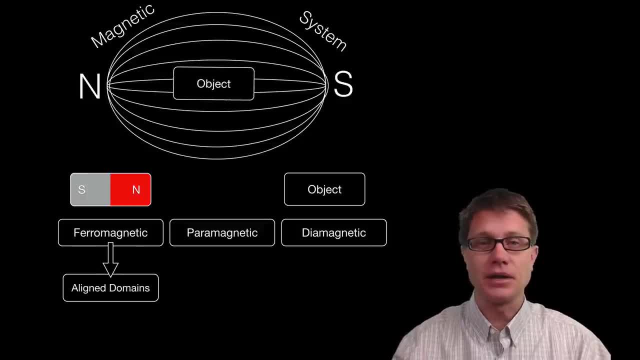 magnets on either side, it will actually be magnetized to the object itself. Now, if you line up parallel to those magnetic field lines And what we are doing is inducing these small fields within the object itself, Now, if you pull it out, even though it is parallel, if 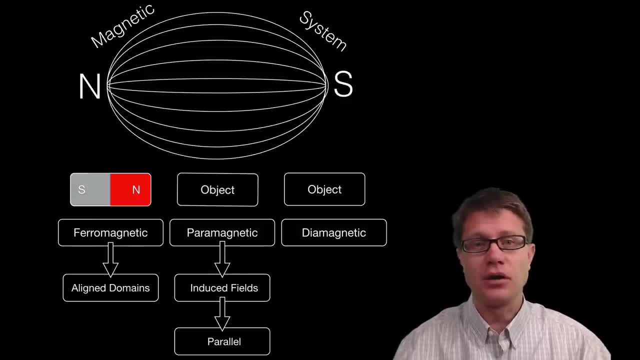 you pull it out, thermal motion is quickly going to scramble all those induced fields inside it. If you put paramagnetic material inside really strong magnets, it will actually be attracted to both the north and the south pole. Now if you take diamagnetic material, 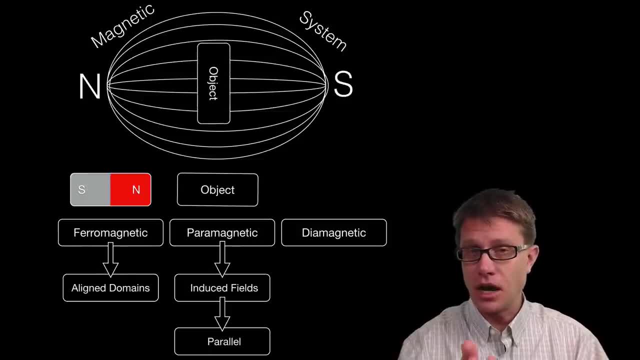 and put it inside a magnetic field, it will actually work in a magnetic field And if you pull it out, even though it is parallel, if you pull it out, thermal motion is quickly going to be in opposition. It still has these induced fields, but it will be in opposition. 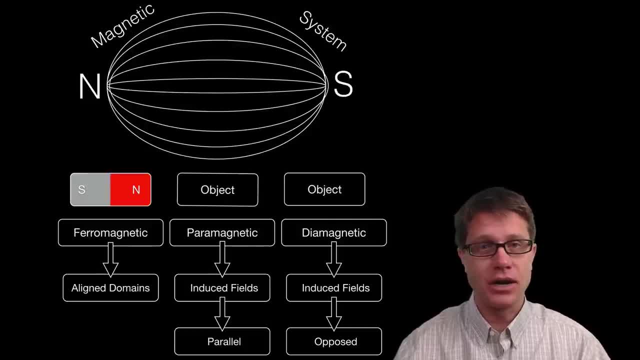 to the magnetic fields. Again, you take it out: Thermal motion is going to scramble all those induced fields and it goes back to being non-magnetic. So why is it that permanent magnets do not do this? Well, they do If you heat up a permanent magnet above what is called 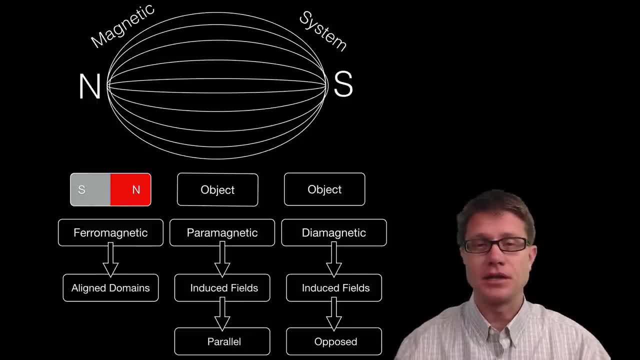 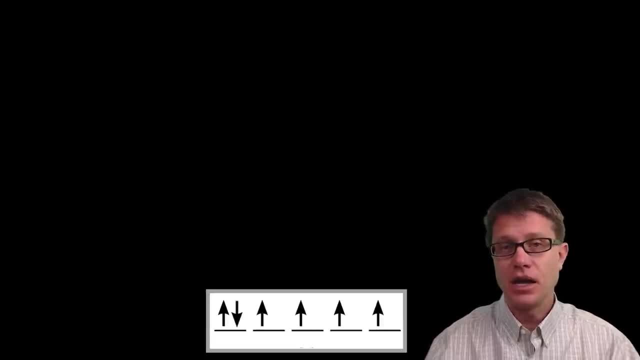 the Curie temperature, all those magnetic fields get scrambled and it is not a magnet anymore, And so this is a quantum property And it is based on electrons. Electrons have a spin And if you have a number of unpaired electrons, you have a number of unpaired electrons. 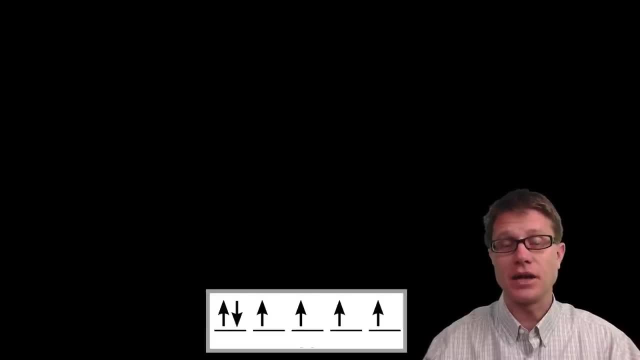 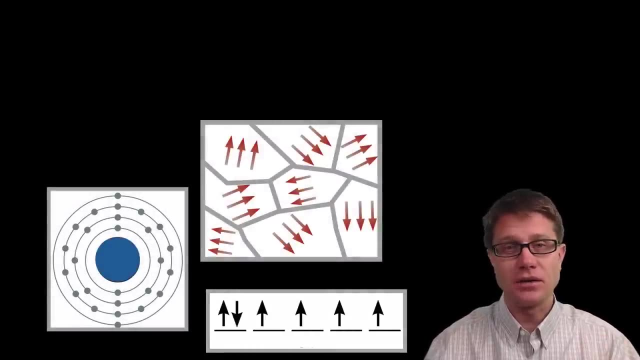 They are not counteracted by the other spinning electron, And so it is a tiny little magnet. And since atoms are made of lots of electrons, atoms are tiny magnets and they will align themselves into domains which are bigger magnets, up to about the size of a millimeter. And 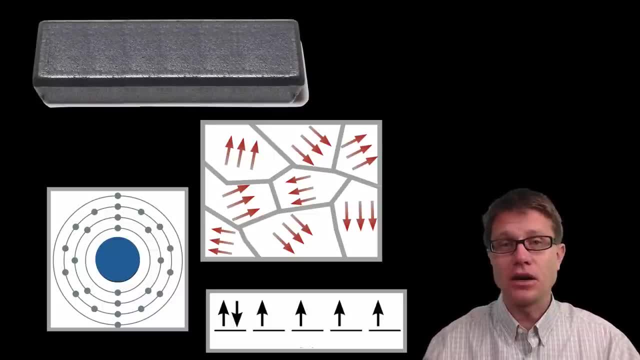 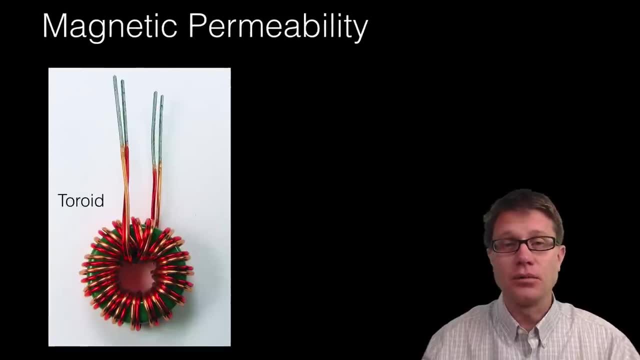 then you can have the whole magnet be magnetized, And so, even though it is a large property, it is actually a quantum property that is responsible for this magnetism. And how do we measure that? Well, we use something called magnetic permeability, And I have made a video. 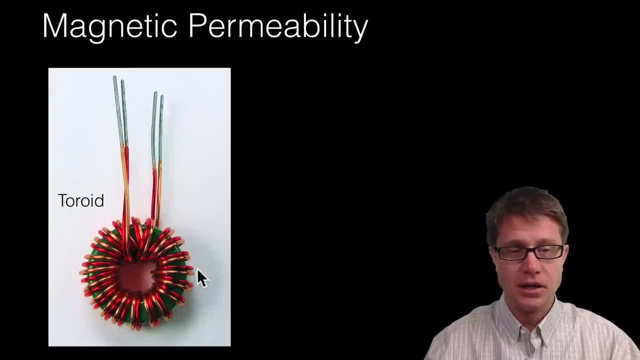 on that already. So essentially what you do is you take an electromagnet. So we could take an electromagnet. This would be attached to some kind of a power source on the other side, And then you can put the object that you want to measure in the middle in this, what is called a toroid. 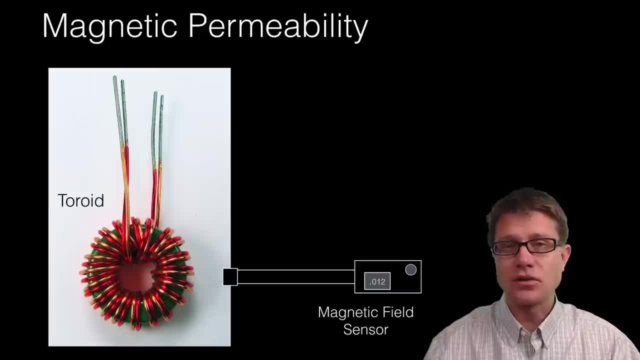 And we can measure the magnetic field using a magnetic field sensor, And so if we were to just place this toroid inside a vacuum, we could measure the magnetic permeability of free space. That is going to be the standard that we will compare other objects to, And 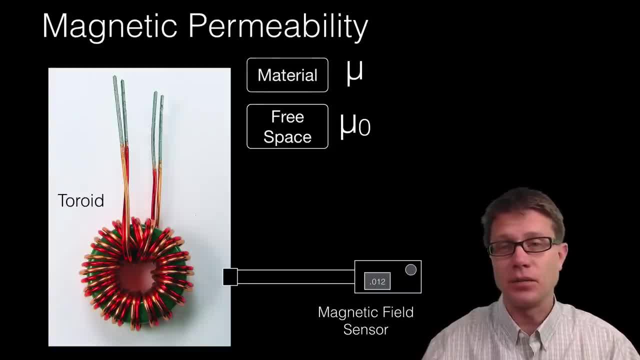 then we can simply put the material inside there and measure its magnetic permeability as well, And so the relative permeability, or mu sub r, is going to be a way to determine if this is ferromagnetic, paramagnetic or diamagnetic, And so this chart should make sense to you. 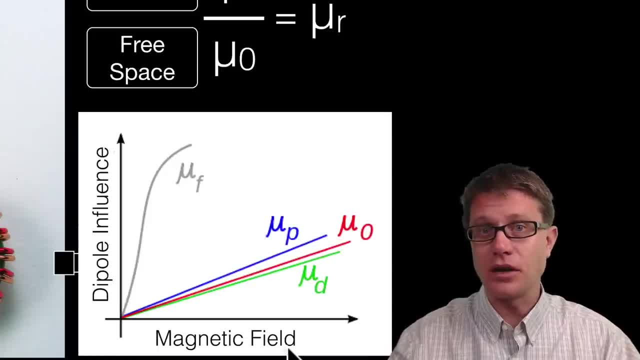 What we are doing is increasing the magnetic field, So we would be turning up the strength of that magnetic field And then we are seeing how the dipoles, or the magnetic permeability, is affected by increases in that magnetic field strength. And this would be the line. 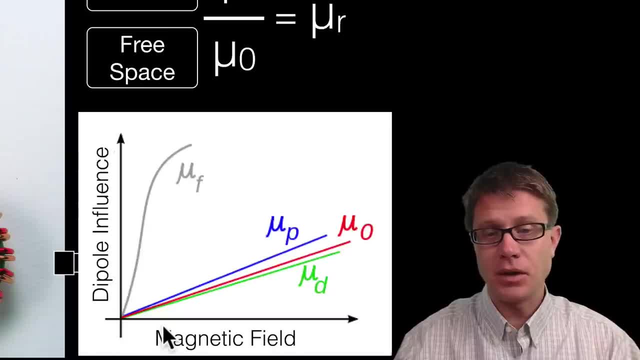 for ferromagnetic material. As we increase the magnetic field, it quickly increases the magnetic field strength And so, basically, all these dipoles align, the domains align and we have a permanent magnet. Now this right here, the red line, is going to be the magnetic 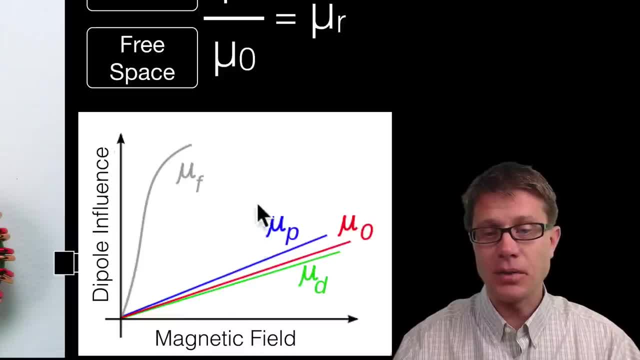 permeability of free space. So that is our standard, And so paramagnetic material are going to increase their dipole influence as we increase the magnetic field. You can see it is a linear relationship, But they are going to be slightly greater than free space. 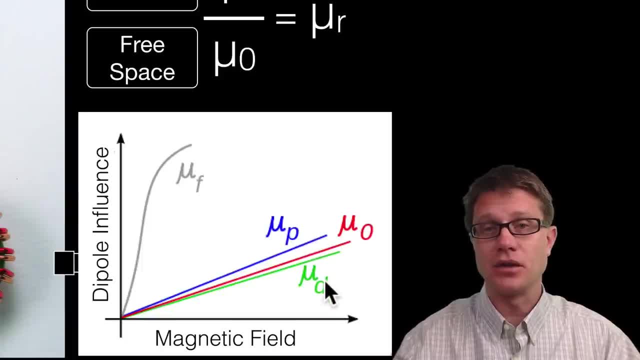 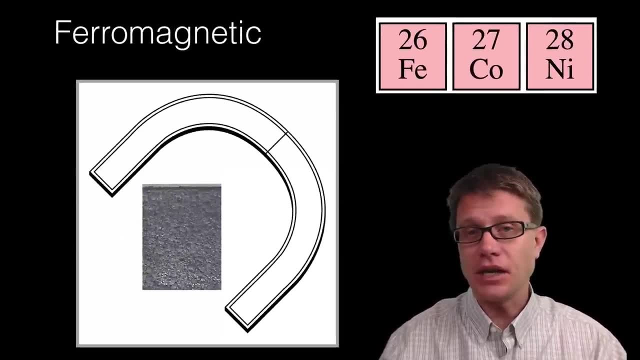 And diamagnetic material slightly less than free space in their ability to be magnetized, And so ferromagnetic material would be like iron, cobalt, nickel. If we take any of these materials and put them inside a magnetic field, so we are going to put them inside a magnet. 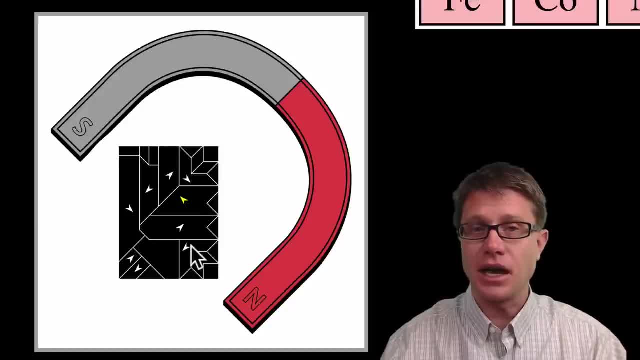 like this. there are a lot of domains or areas inside that ferromagnetic material where they are all pointed in the same direction. In other words, all these tiny magnets are lined up, But if we put them inside a magnetic field like this, watch what happens to those domains. 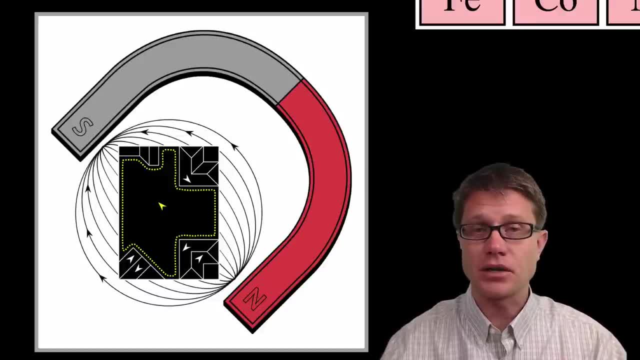 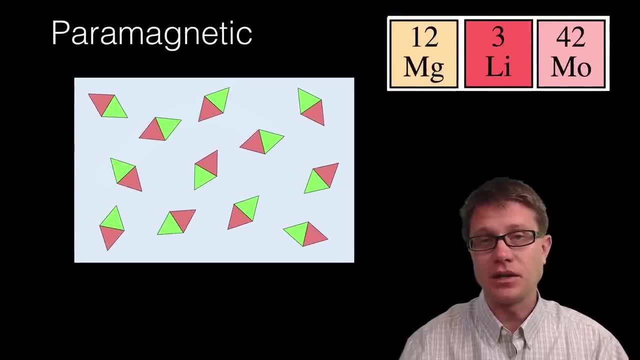 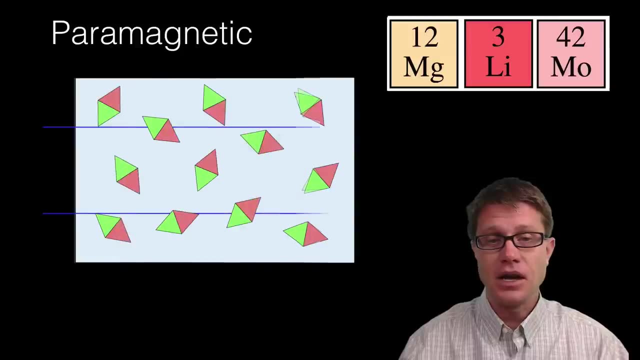 They grow in size and they all start to point in the same direction. So now what you have created is a permanent magnet If it is a paramagnetic material- so, example, magnesium, lithium, molybdenum- if we put those inside a magnetic field, it is also going to have these tiny little fields and they 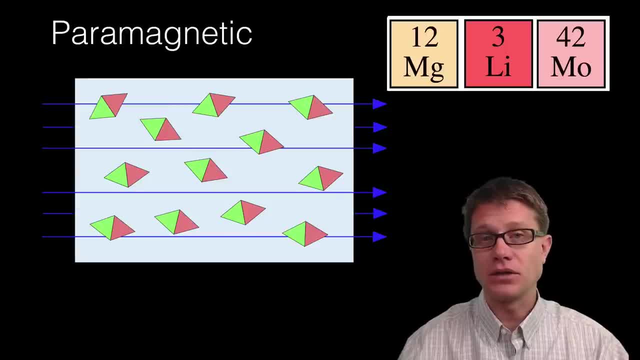 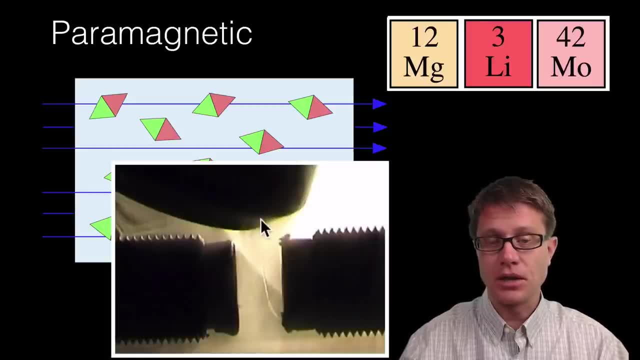 are going to start to align parallel to that material, And so if we have a really, really strong magnet on either side, and right here they are dropping, this is liquid oxygen through the middle. Liquid oxygen is paramagnetic, And so it is actually being attracted to one. 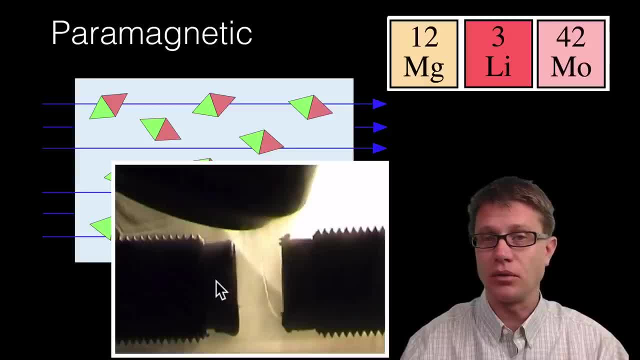 of these poles. So if we were a little closer to this side it would be attracted to this pole over here. Now, once it falls through, if it does not get attracted to one of those poles now, it goes back to being just regular material again. It does not keep that magnetic field If we 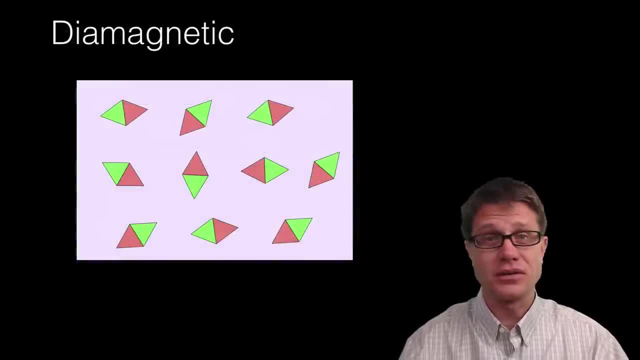 are looking at a diamagnetic. so what is that going to be? That is you, But it is also like wood, it is water, it is pretty much everything you can think of that does not have all these unpaired electrons. that is diamagnetic. So what happens if we put that inside a magnetic? 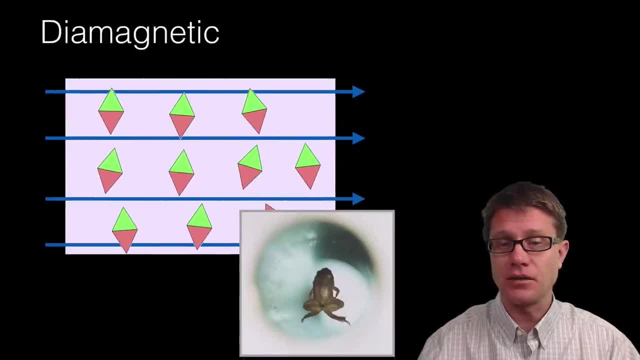 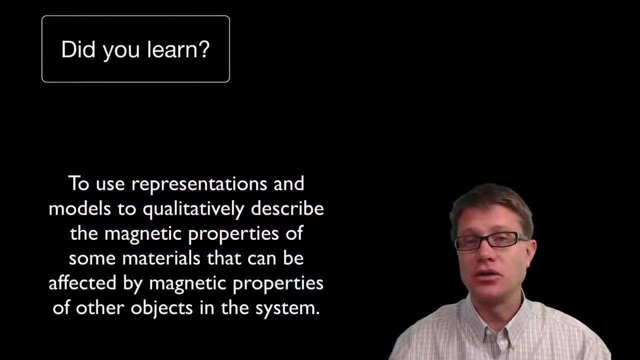 field, It will actually work in opposition to those magnetic fields, And so since this frog is diamagnetic, it is kind of being pushed away by these magnetic fields, And that is a greater push than we have just from gravitational field strength. So we get this levitation, And so did you learn to use representations to figure out. 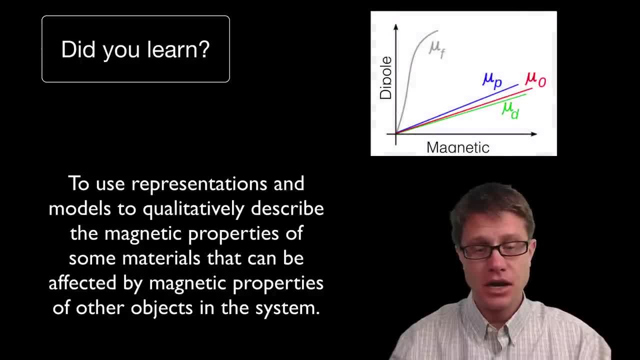 how different materials respond to magnetic fields. Again, they could be ferromagnetic, quickly responding and becoming permanent, Or they could be paramagnetic, so they are going to align with it, Or diamagnetic, so they are going to align with it. So they are. 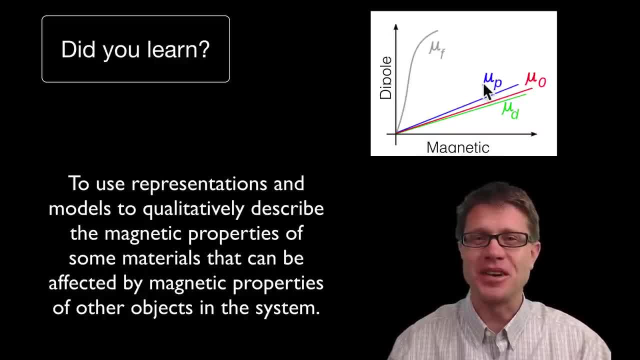 going to align with it, And so this is what we are going to do. We are going to put this thing without it. So hopefully you learned that And I hope that was helpful.